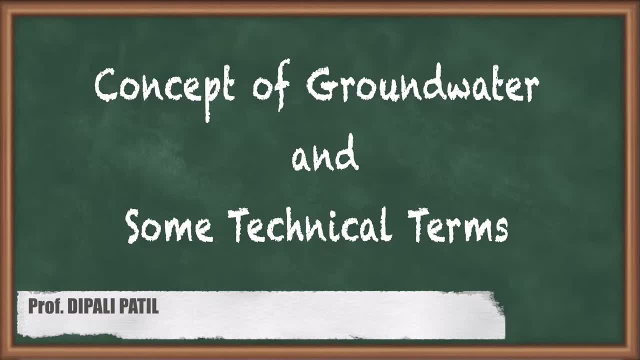 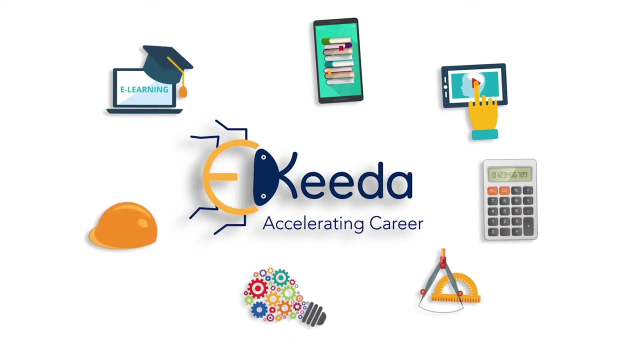 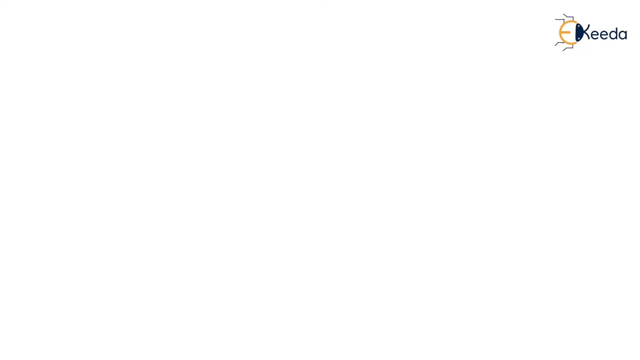 So we are dealing with all the parameters which are flowing above the surface. Now it's time to calculate, or determine the groundwater and its characteristics. So in this chapter we are going to study the contents which are included in this chapter is: 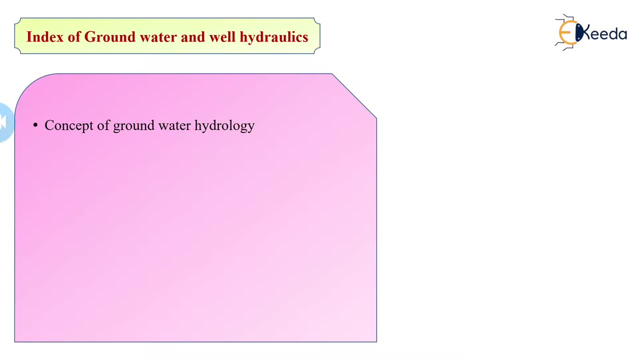 concept of groundwater hydrology, definition of aquifer, aquitard and aquifuge. then occurrence of groundwater well, hydraulics, that is, steady state flow in a well. then equilibrium condition or equation for unconfined aquifer. equilibrium equation for confined aquifer. then the test which are required for the aquifer. then design of the aquifers. 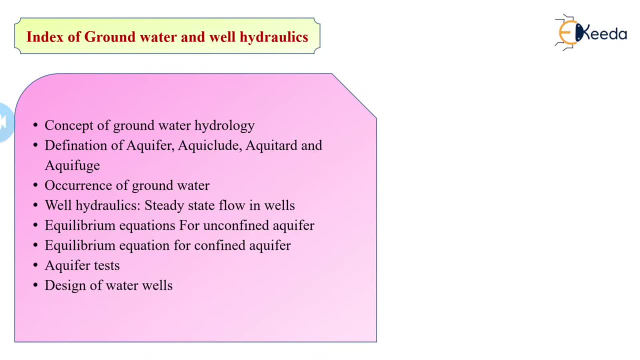 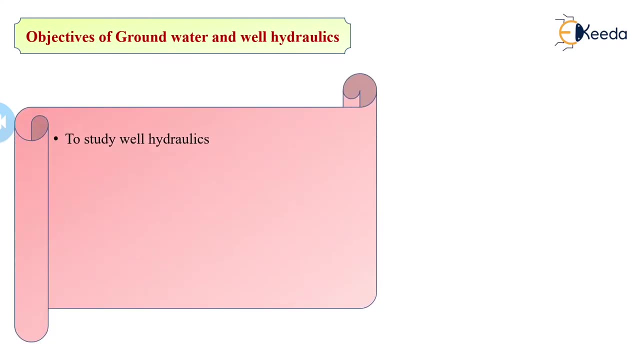 Then design of the aquifers, water wells and the numericals. So these are the contents which are included in this chapter. So main objective of this chapter is to study well hydraulics, then to study steady state in well, to study equilibrium equation for unconfined aquifer, to study equilibrium equation for 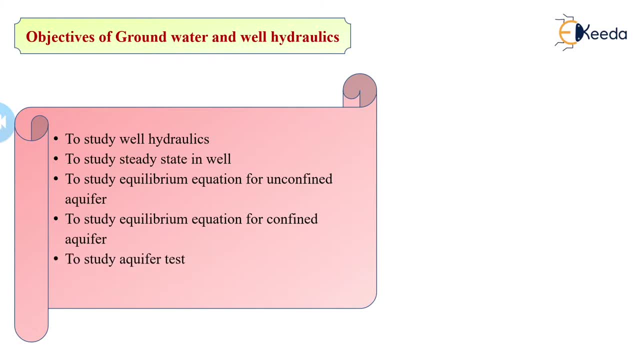 confined aquifer, then to study aquifer test and to study yield from the well. At what manner? and by using this equation we are going to find out the yield or the discharge through the well. After completion of this chapter, student will able to explain. 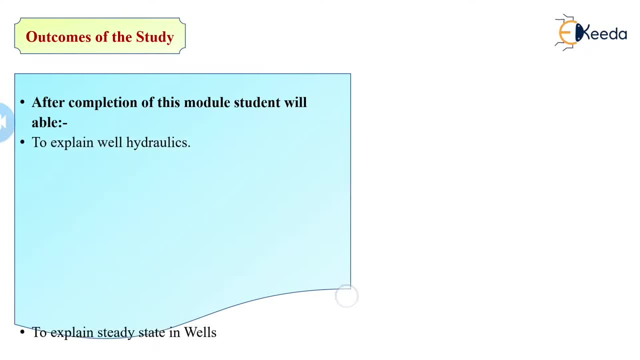 well hydraulics. they will able to explain the steady state in the well. they will able to derive equilibrium equation for unconfined as well as confined aquifer. they will able to explain various aquifer test and they will able to explain the yield from the well. 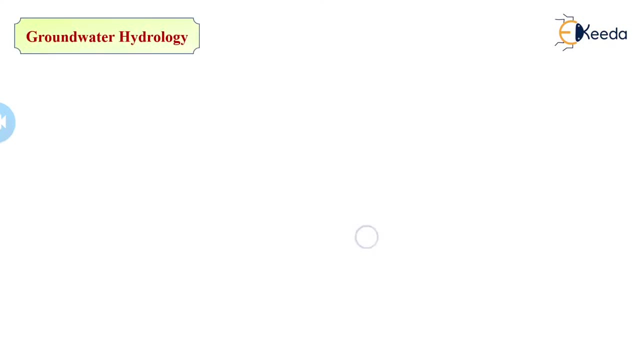 Now let's start with our first concept or first content, that is, groundwater. hydrology, See, it is the science of occurrence, distribution and movement of a water below the surface of the well. So let's start with the first concept or first content, that is, groundwater. 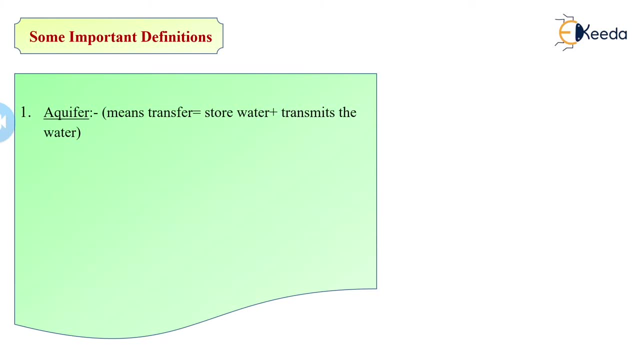 pervious formation. through the pervious section, the ground water again, or the level of the ground water, will starting to fill this aquifer or starting to fill the area of a well so that we can easily extract the water through this open surface area. so it's, it means that it stores the 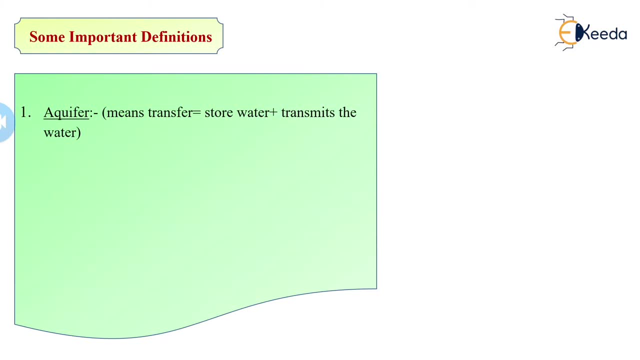 water as well as it is able to transfer the water, hence it is known as the aquifer. so again, if we want to define this aquifer, so these are the permeable formations having structures which permit appreciable quantity of a water through them under ordinary fill conditions. so thus these 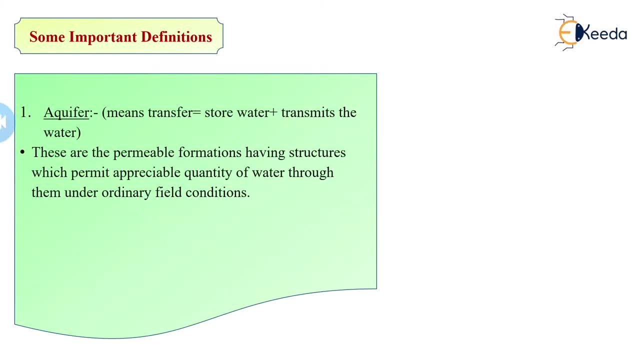 are geological formation in which ground water occurs, For examples of the tanta in trebles. we need that the sand and grab Pleas are the permeable one, permeable the voids and the gaps between the two particles of the side and grabber these two high or a distance is. It is not so true this way, through this course, water is. 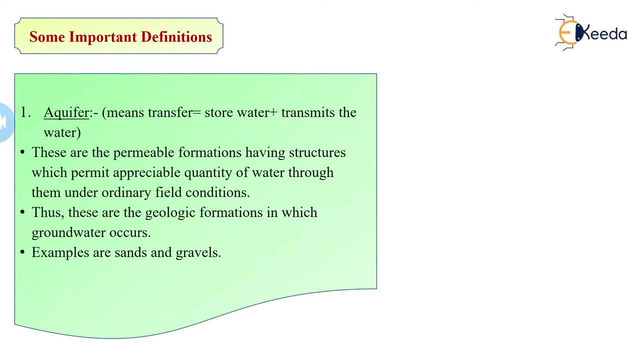 easily passed through or water will easily flows down. so this is the permeable formation. so if such type of of a soil, if such type of a geologic formations are there and in this geological formation, if we construct the well or we construct the any two well, 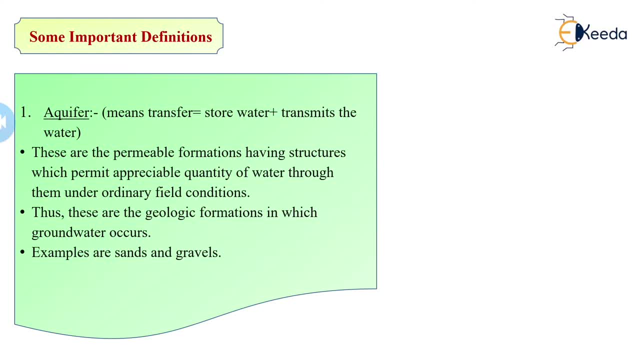 then it is termed as a aquifer, which stores the water as well as which is used to transfer the water is known as a aquifer. it transmits the water. it is known as a aquifer. so I hope you understand this phenomena now in this we. 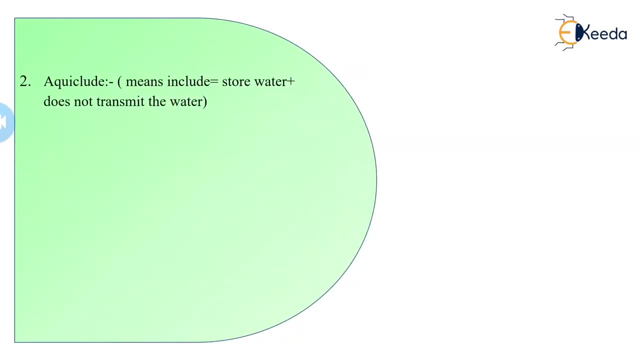 have a second parameter that is actually clued. so if we divide this word, actually clue, actually plus clue, or it means the include. include means what it stores the water but it does not transmits the water. the epic clues are you, the impermeable formation which contains the water but are not capable of transmitting. 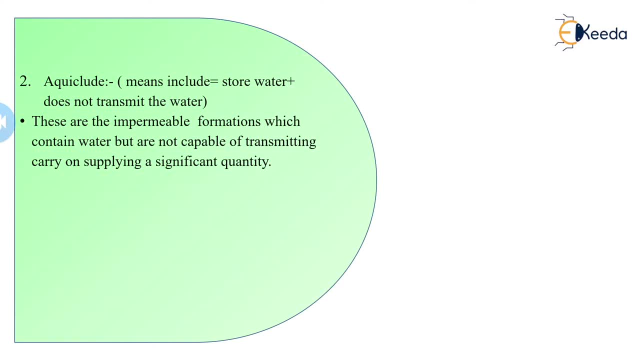 the water and supplying a significant quantity, It is not able to supply this water further in the downward direction. So we have the example for this Example, for this is clay, So clay. we know that the particles between these two particles in the clay, the soil particles, 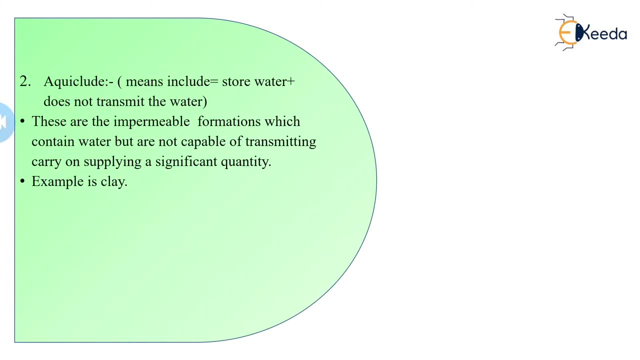 the distance between these soil particles are two less. So through this the water will not easily pass, or water will not easily transfer in the downward direction. So it stores the water. Its characteristic is to store the water, The capacity, or until the voids and pores will fully. 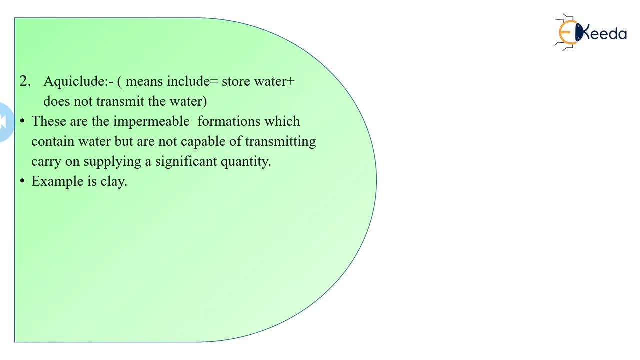 get filled with water. So the water will not easily pass or the water will not easily transfer. It is filled with the water up to this level. This type of a soil, this type of a geological formation store the water, but it is not able to transmit the water. Hence it is called as a 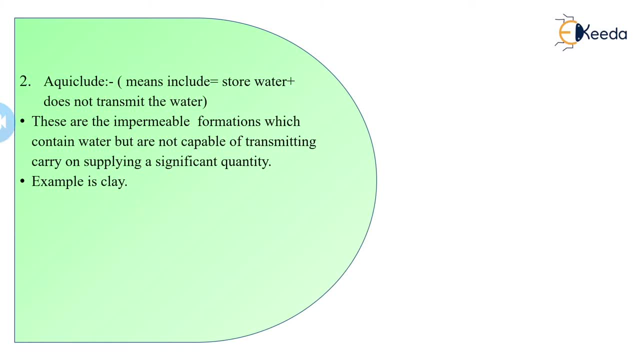 aqueous fluid. Then we have the second parameter is the aqueous fluid. Aqueous fluid means what? Aqueous plus fluid means confused. Why it is confused? See, it becomes like that sometimes the water which is having impermeable formation, but this 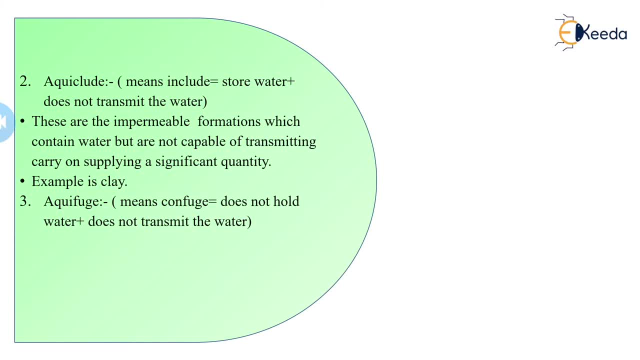 it does not contain the water and does not allow this water to transmit. below Why it is happening, See: 90% of all developed aquifers consist of unconsolidated rocks, chiefly gravel and sand. Sands are composed of a microscopic particles. 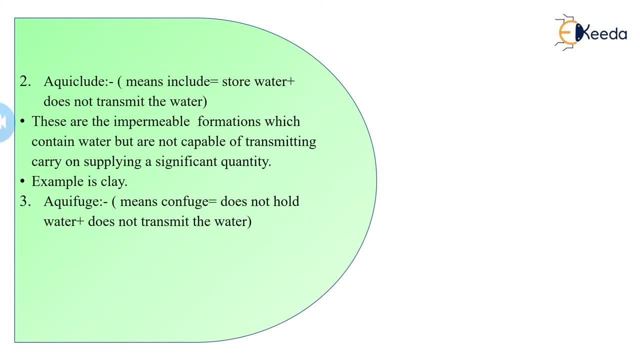 that are rounded. They are called as aqueous fluids. They are called as aqueous fluids. They are rounded or angular in shape. We know that They drain easily, do not swell, possess insignificant capillary potential and, when dragged, exhibit no shrinkage. 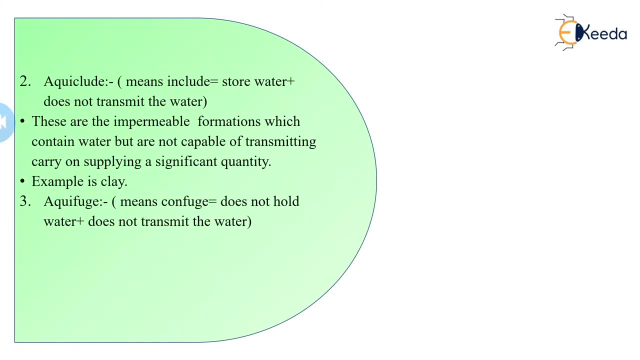 Clays, on other hand, are composed of a microscopic particles of plate-like shape. They are highly impervious, exhibit considerable swelling, possess a high capillary potential and contain a considerable volume reduction upon drying. So hence it consists of two types of or. 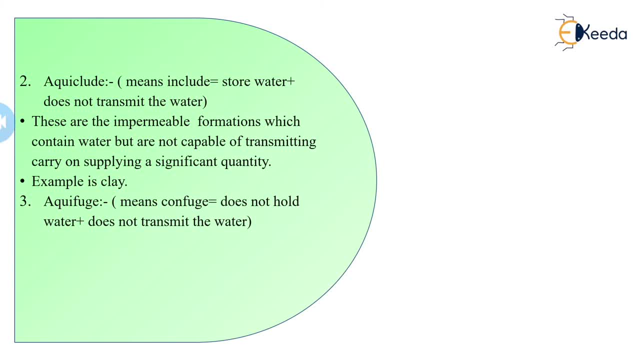 it consists of the mixture of the impermeable plus the impermeable formation. Hence it gets confused, Hence it is known as a aqueous fluid. It is the impermeable formation which neither contains the water nor transmits any water in the downward direction. So we have 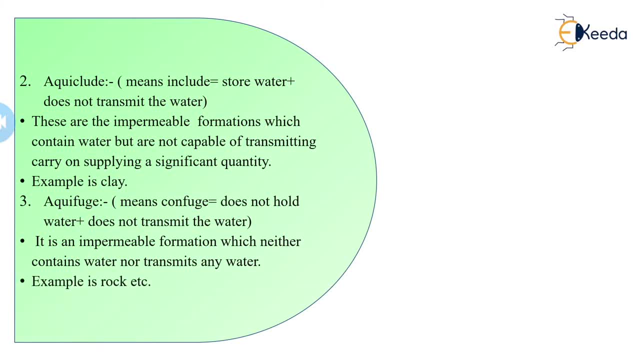 the example of rock, So sometimes rock, the fissured rock or sedimentary rock. that type of a rock has a tendency to store the water in less amount. But what happen if there is a fault? there is a fissure on the rock surface and the rock is a sedimentary one? 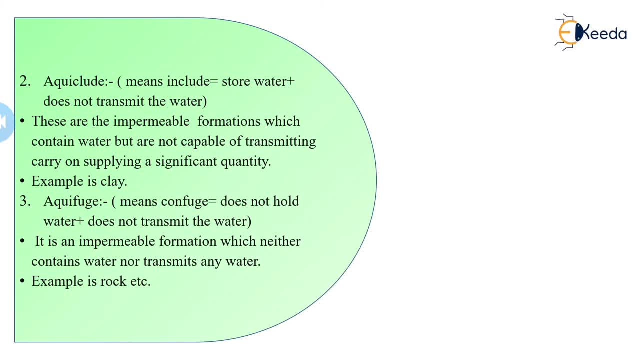 So what happens? because of the continuous application of the water through this crack, through this fault, The water will get absorbed by the rock, So this is called aqueous fluid. Sometimes will get stored in the type of geologic formation. but what? after some time, or 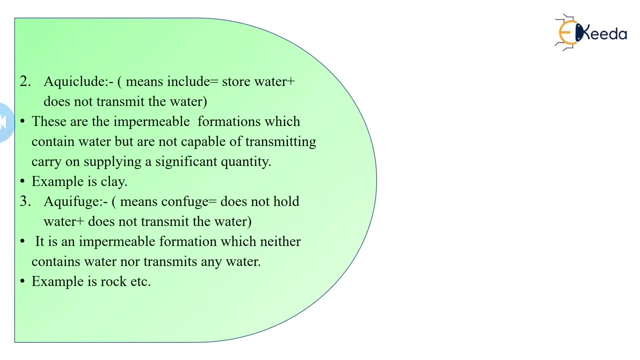 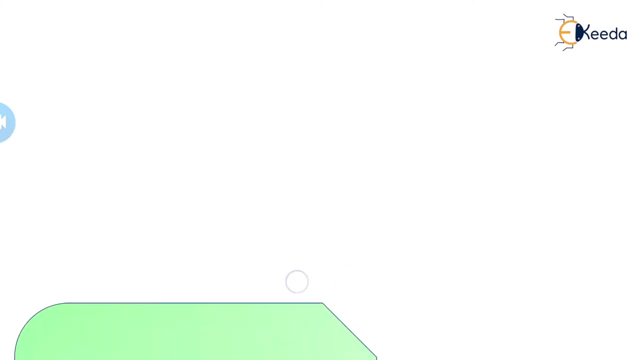 after some period this contains and this amount of the water will get discharged away through or from the from this type of a geological formation. so hence it is called as a at the future. that means what? it does not hold the water and does not transfer the water anymore. so our next parameter is actually start, see, 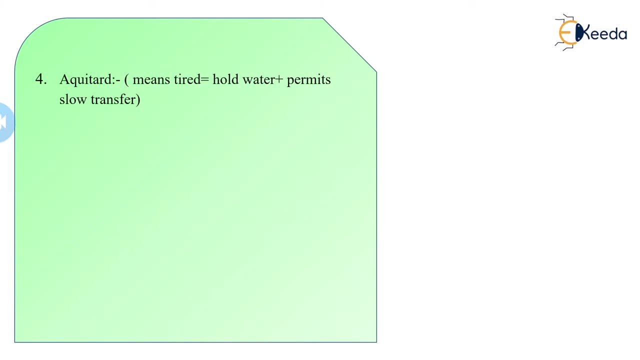 actually first start, or we can say that it's tired up, continuous or taking. because of the in taking of a continuous quantity of a water, it becomes star, so it means that it hold the water but permits the water at the flow rate. so because of the continuous in taking this type of 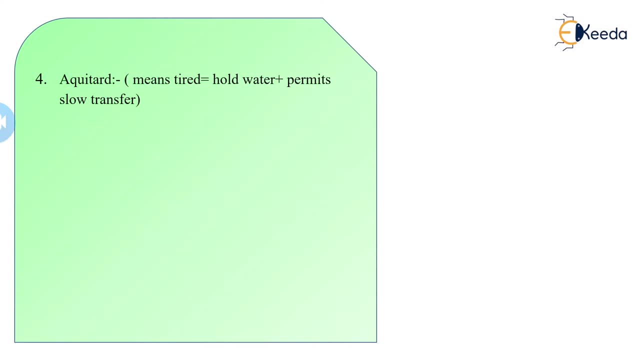 geological formation will get tired and hence it does not allow the as the higher quantity of a water in the further downward direction. hence it is called as a at with that. so it is again impermeable formation which hold the water but transmits the water at a flow rate. an example is the silk. 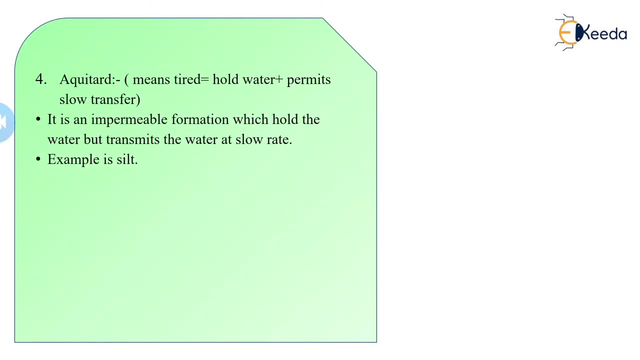 silk particle. that is the finest the particle of a soil. if the more or finest particle of a soil, the week comes together it becomes a state. so the said it is carrying capacity or it soaring surpass capacity is good but it does not allow, like clay, it does not allow the clay totally avoid the 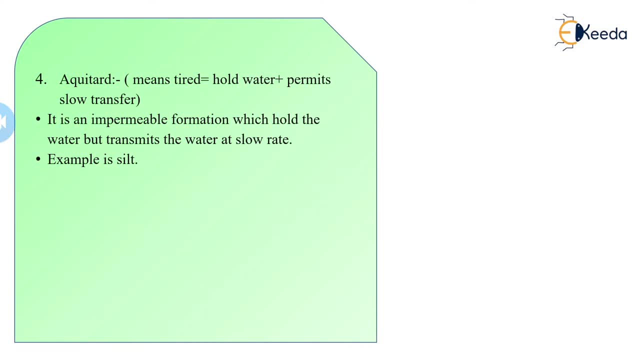 transfer of the water, but said at least to some amount and least less amount of a water will be transferred, but at the slow rate in the downward direction. so these are the some of the important parameters of definition related to the attributes we have the accuracy at refer. a quick nude. 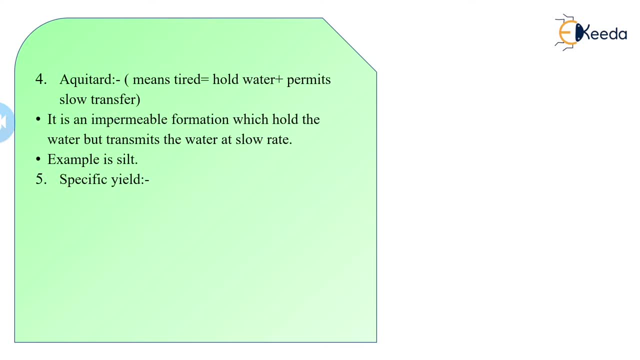 then we have to actually shoot and we have the actually done, then the specific end end means what the capacity of formation, that is, see, the capacity of a formation to contain water is obviously measured by porosity, how much quantity of a water that can be taken by the particular soil, particular surface. this 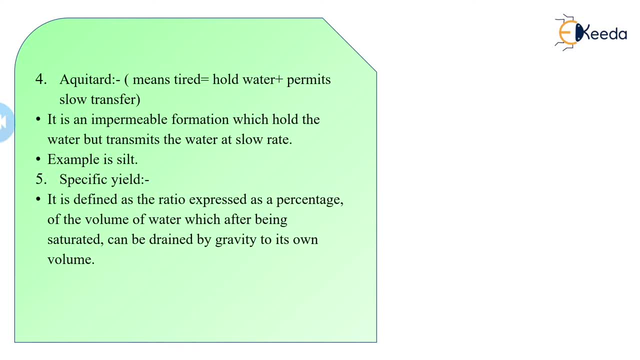 can be calculated by its porosity. so the high porosity does not indicate that an aquifer- for I prefer- helps to transfer the amount of a water to the well or to any other extracted area or to any other the underground surface area. the only water which can be obtained from the aquifer is that which will flow by gravity only. 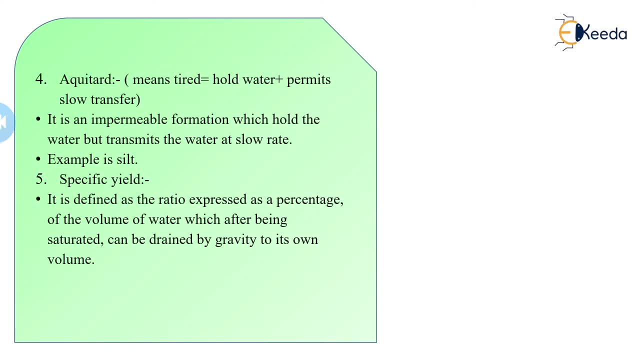 hence the water will be transferred to the well. and the water will be transferred to the well, so the other, the more surface area, will be transferred to the well. hence the specific aid is defined as the volume of a water which, after being saturated, can be drained by gravity to its own val volume, and it is expressed 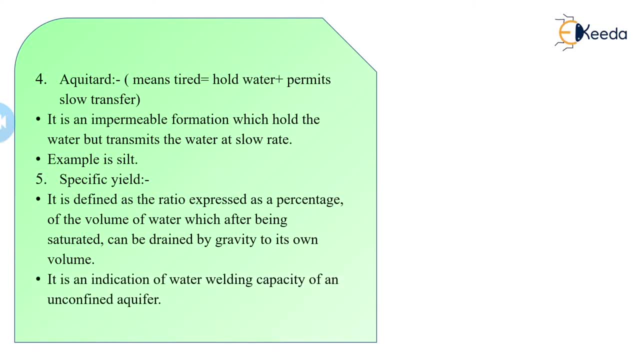 in a percentage. see, it is an indication of a water welding capacity of an unconfined aquifer, so it can be found out by using the exact amount of water, that is, just the water that is entering the water and then also going to be ran on. 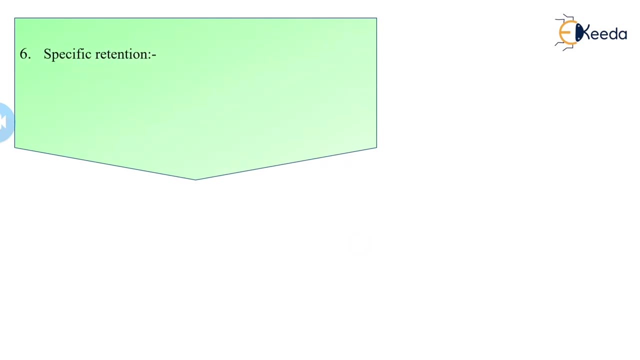 the ground and the water that is entering the ground has to be drained from the ground. that is specific. it is equal to volume of a water drain by a gravity only divided by the total volume into hundred. so this, from this we can easily find out the yield of a well: specific yield of a well. specific retention: see specific. 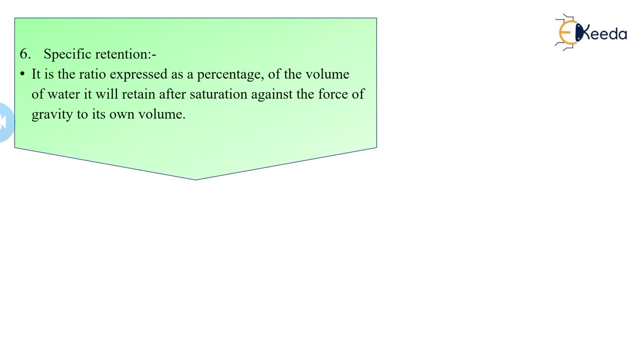 yield is always less than the porosity, since some of water will be retained in the aquifer by molecular and surface tension forces. hence the surface retention is defined as the volume of a water that it will retain after saturation against the force of gravity to its own volume is known as the. 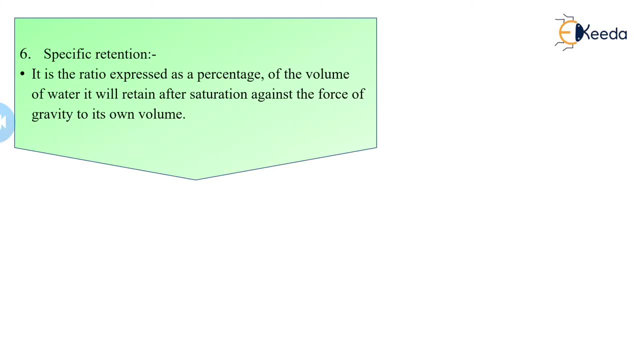 surface tension and the value of a specific L depends upon the grain size, shape and distribution of a pores and compaction of a stratum. so according to the grain size, shape of the particles, then the distribution of a pores and the compaction factor, only the specific rate depends and on the 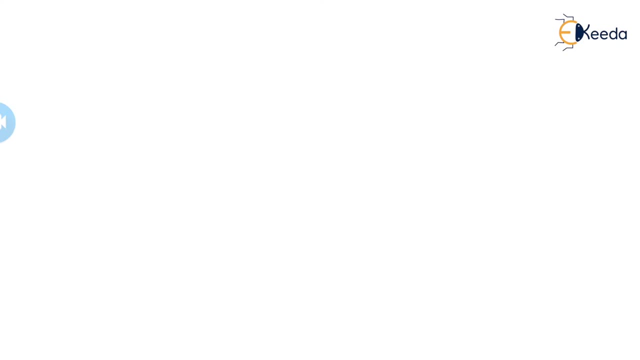 specific rate the retention will depend. so the amount of the water which is retained, which is left out in the part of a aquifer that cannot be extracted or that cannot be flow under the gravity of a flow, that part of a water divided by the total volume is, gives you the surface retention. 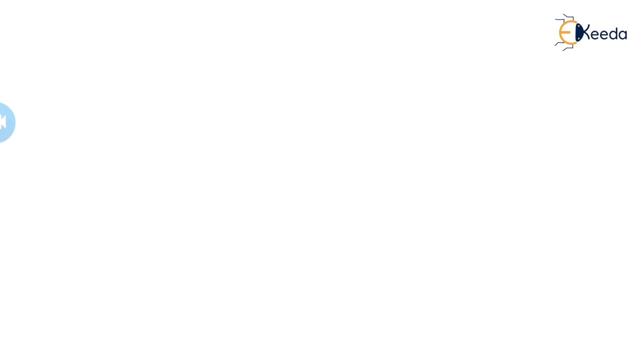 or specific retention. so these are the some of the important definition that might be useful for the uh, you, you, for the calculation of the numerator. then the storage coefficient, one of the parameter, important technical parameter. we have that storage coefficient. it is defined as the volume of a water that an aquifer releases from or takes into a storage per unit surface area of. 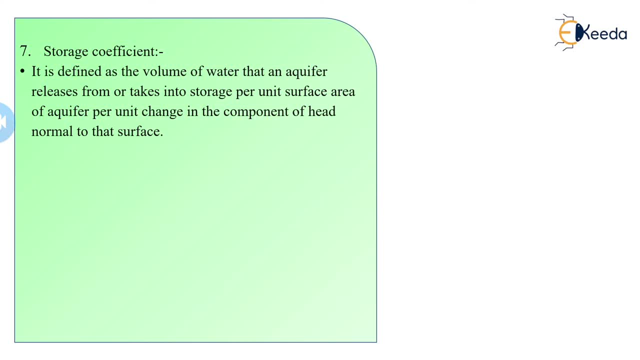 aquifer per unit. change in a component of of a surface area of aquifer per unit. surface area of the water because of the volume of the. this the volume of the solution Wis Kerr takes into storage per surface area. the surface area of the aquifer per unit. 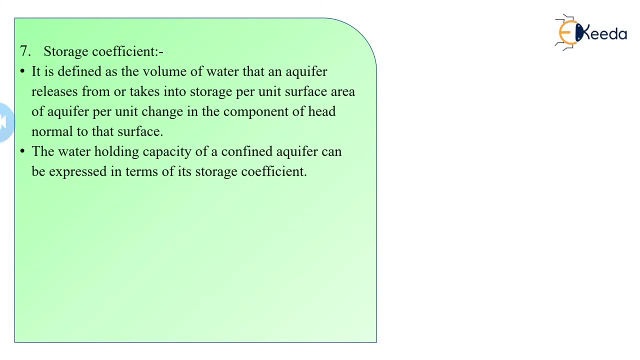 change in the component of the head. if we have initial level of a water and after some time, or after extracting the level or at extracting some amount of the water, this level will depressed. so this depression according to this component head of the change or according to the surface area of the 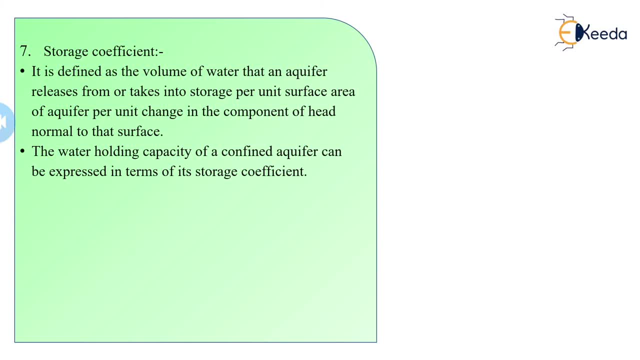 aquifer. the volume of water at releases through the aquifer is known as the storage coefficient, so it is the water holding capacity of the confined aquifer. its can be expressed in the terms of a storage coefficient only. this value of storage coefficient ranges between 0.75 to 0.25. 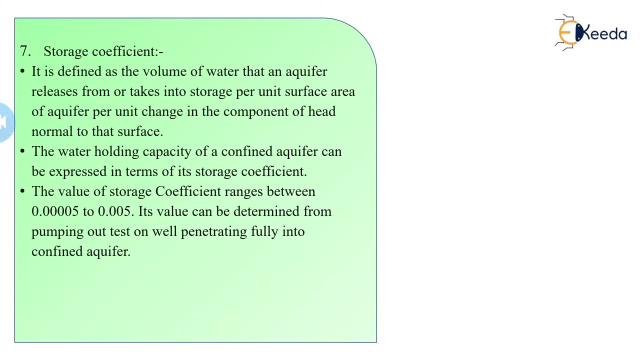 0.00005 to 0.005.. Its value can be determined from pumping out test on well penetrating fully into the confined aquifer. The storage coefficient for an unconfined aquifer correspond to its specific yield. It is equal Storage coefficient when we are dealing it with in. 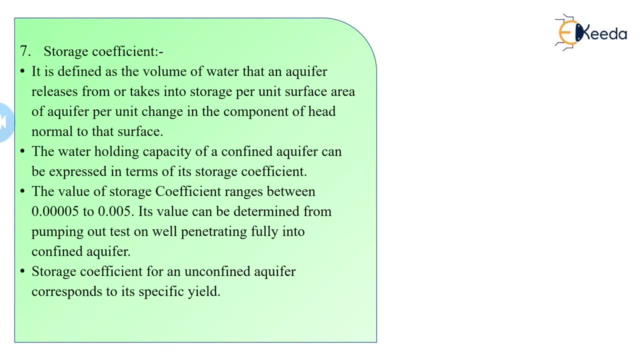 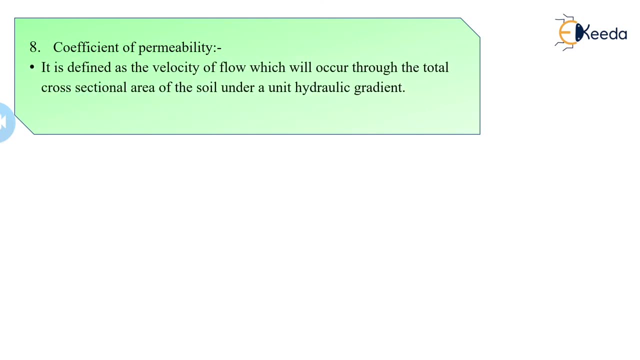 terms of an unconfined aquifer. the storage coefficient. it is nothing but a specific yield and it is denoted by the s. Then we have the coefficient of permeability, one of the, If you remember that in geotechnical engineering also you are dealt with this terms, this technical terms, Goefficial permeability means it스터ph eresis. Alright, let us continue. So here we are going to step back and try to reasonably, if, form the second part of the manga, So the third part in favourite, one where we have 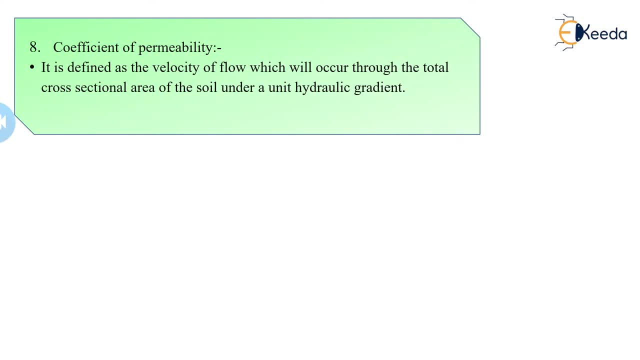 is defined as the velocity of flow which will occur through the total cross-sectional area of soil under a unique hydraulic gradient. This gives you the permeability constant, or this gives you the permeability rate coefficient gives you the at which velocity or at which rate the flow will occur through the total cross-sectional area of the given soil sample. 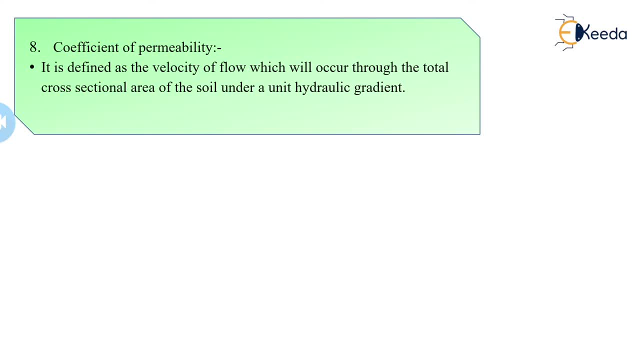 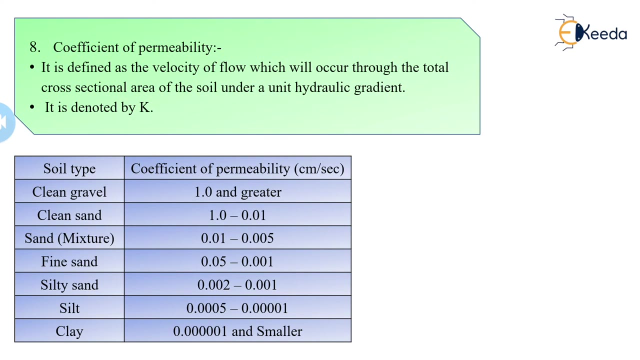 or the given geological formation under a unique hydraulic gradient. It is denoted by K, See some of the soil type are given. here is when the gravel is there, the coefficient of permeability K value is 1 or it's greater than 1, then the sand is there: gravel and sand it is. 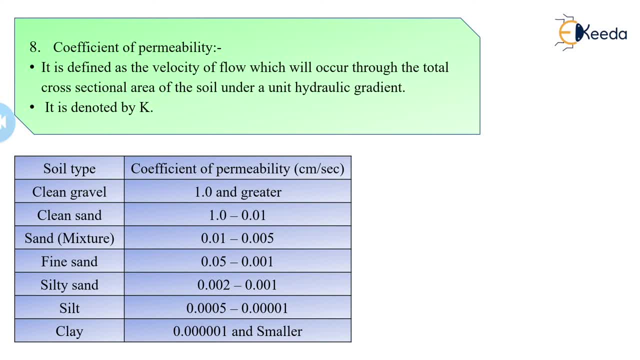 nothing but a permeable formation, this called as a aquifer. So if the aquifer is there, the your coefficient of permeability is 1 or 0.01 to greater than 1. we can say that If the sand is having a mixture, the coefficient of permeability ranges. 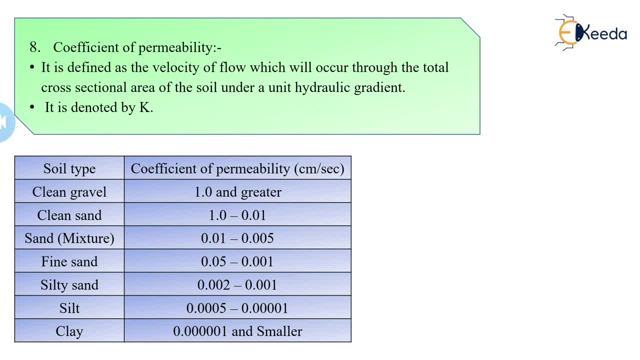 from 0.01 to 0.005.. We have a fine sand, then 0.05 and 0.001, the silty sand 0.002 to 0.003.. Silt 0.0005 to 0.00001, and if we have a clay that means we have a acriclute, then the 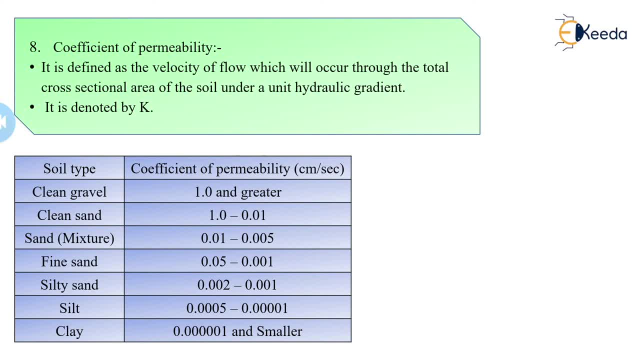 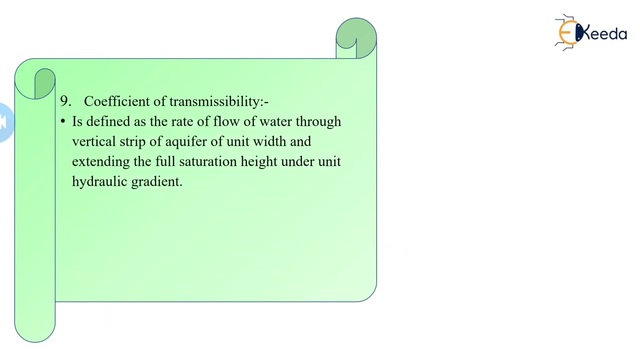 coefficient of permeability is 2 less, that is, 0.0000001, and sometimes it is the smaller than this value. So these are the some of the type and these are the coefficient of permeability. Then we have coefficient of transmissibility: See. the coefficient of permeability gives. 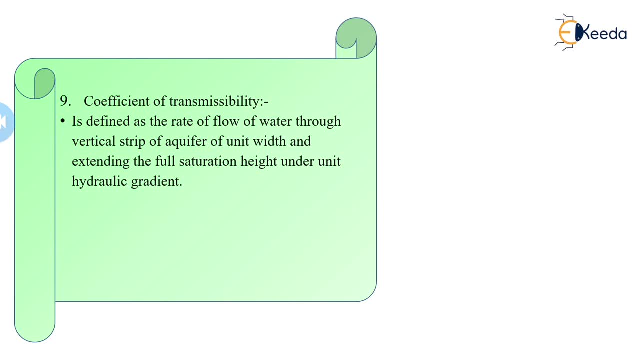 you the permeability, if they give you the permeability constant, for permeability value is the type of a soil. is that so? the permeability constant and permeability value is this. The coefficient of transmissibility means what it is defined as the rate of flow.